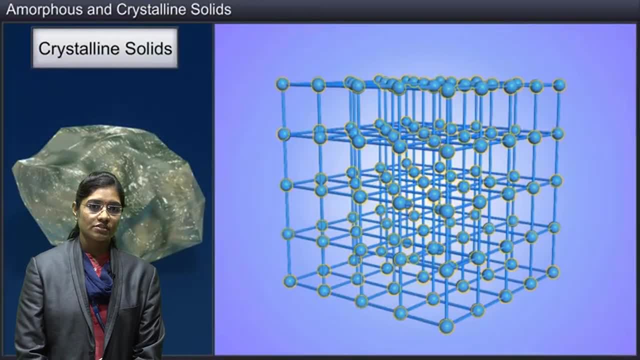 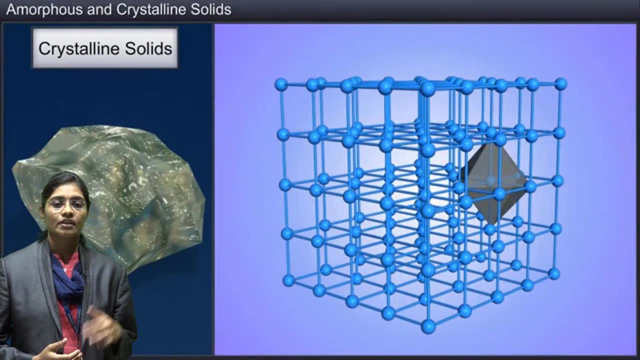 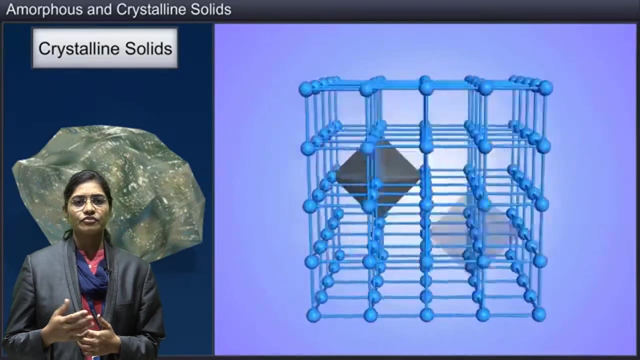 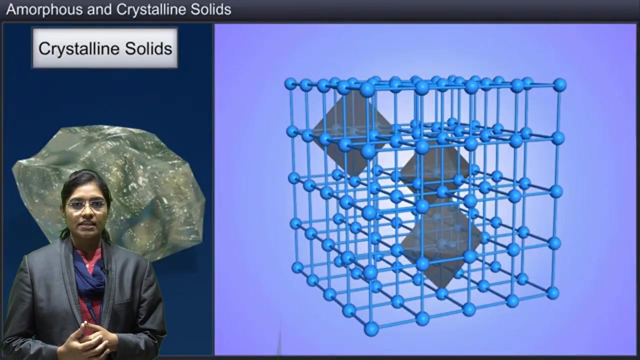 to crystal and solid. So what is crystal and solid? Crystal and solid means the constituent particles like Ions, molecules, atoms are arranged in three-dimensionally in such a way that in a definite order it is a crystalline solid. So if you can see in example, sodium chloride, diamond, graphite, 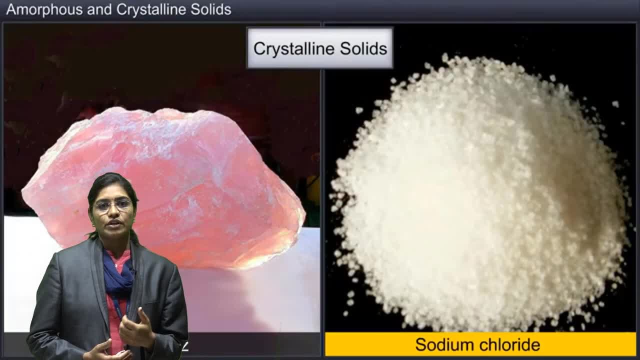 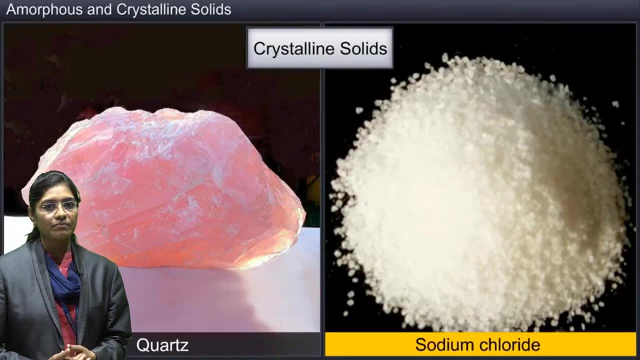 and sugar. If you can see in a sodium chloride, in that sodium chloride salt having a particular arrangement of particles. Also in diamond we can see the arrangement of molecules in a particular order and in same we can see in sugar and graphite also. 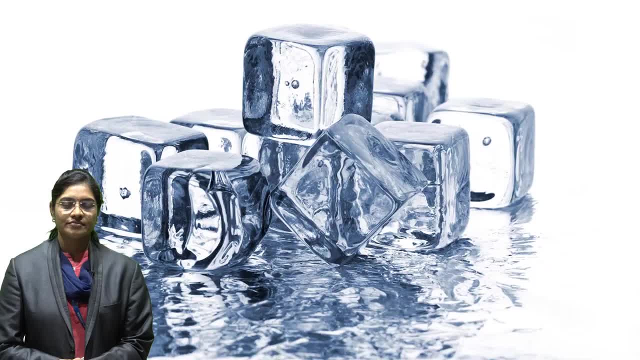 In such a year. we take example of a. here we can see the example of liquid. If you allow a liquid to cool down slowly, that time the liquid is the constituent particle of liquid, arranged themselves in order to see the other molecules. So we can see the in particular. 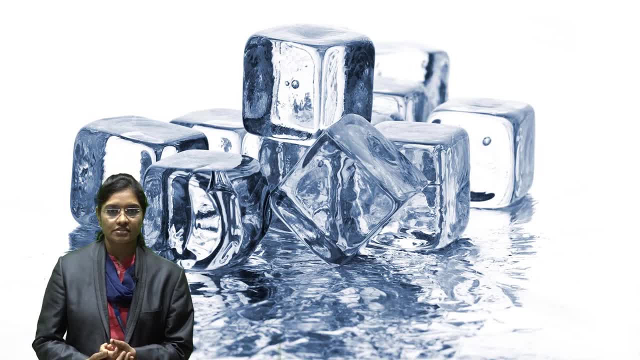 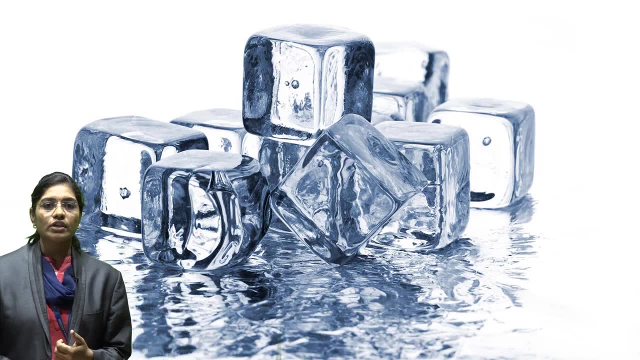 in order, very ordered fashions, that is nothing but a crystalline solid. if you can see the example of water, when we allow water to cool down, what we, what we form, the ice will form and all of you know that, the ice having a constituent, particles in a definite order and is nothing but a crystalline. 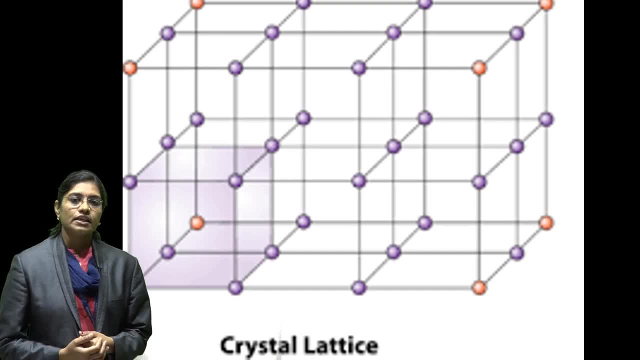 solid. so now we can see the crystal structure. you know that the crystalline solid is made up of, made up from a crystal. so the crystal structure means the arrangement of atoms, ions and particles in three-dimensionally, in a space we can see in a microscopic level, and it is called as a 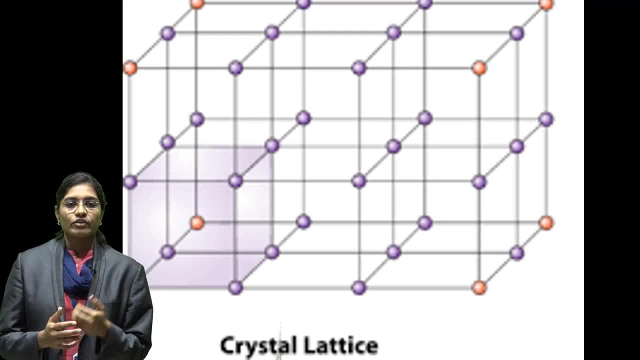 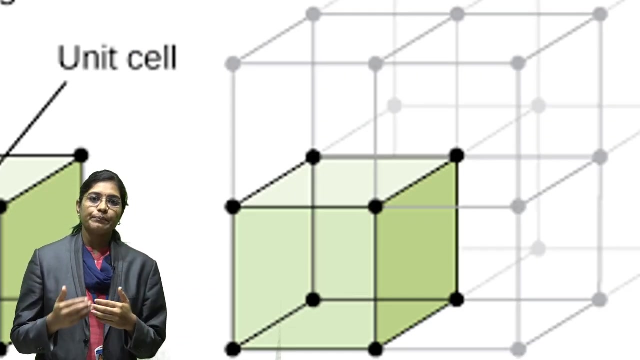 crystal structure. this crystal structure, we can see the unit, say space lattice and agesis. so crystal lattice means the arrangement of ions or particles in a point in a space. it is a crystal lattice. and the unit cell is the smallest repeated unit, the smallest repeated unit of a crystal structure. it is a unit cell. let's see in this figure, this figure: 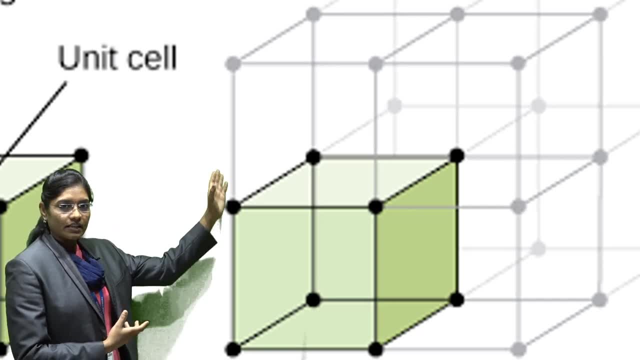 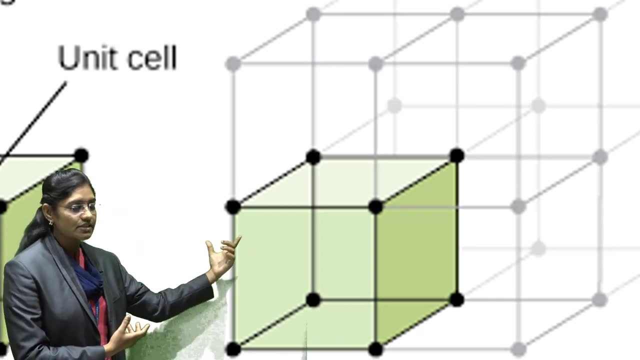 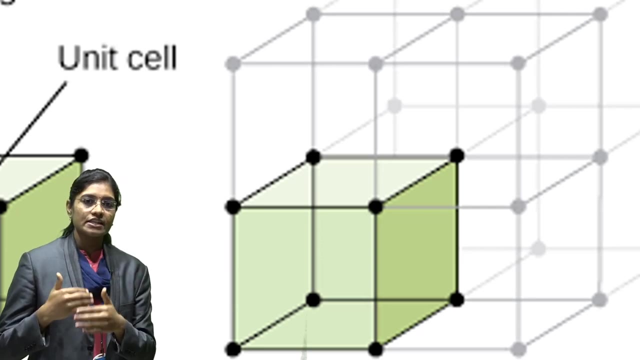 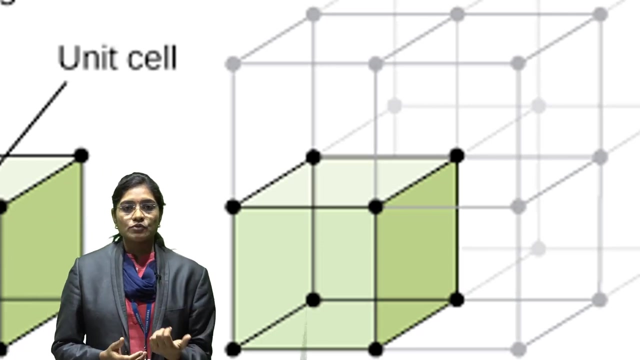 we can see the unit cell here. here is the unit cell in a repeated form. here also this cell is a repeated. here also this is a repeated. so the repeated continuously, the repeated pattern is a continuously in a smallest pattern it is called as a unit cell. so our next. we can see the types of crystal. 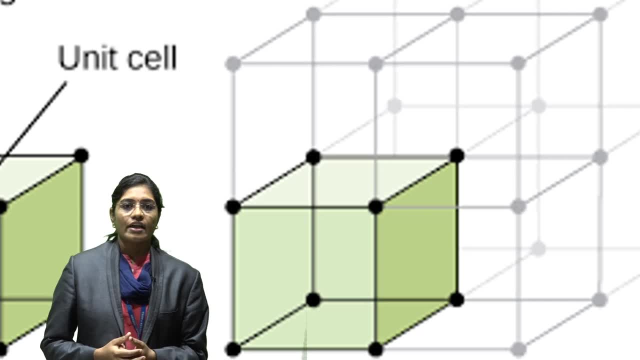 structure. okay, here that crystal structure having four types, such as crystal structure, having four types, such as crystal structure, having four types, such as unit- simple cubic crystal structure. unit. simple cubic crystal structure. unit. simple cubic crystal structure. body center- cubic crystal structure face. body center- cubic crystal structure face. 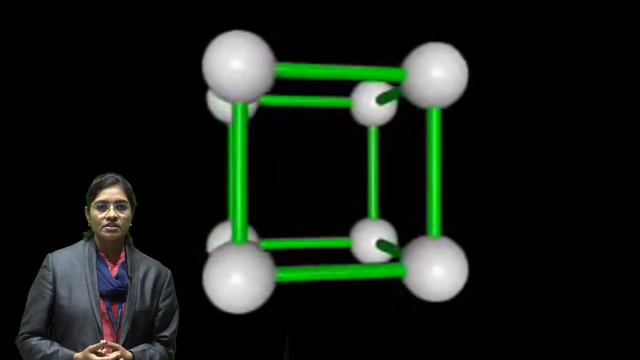 body center cubic crystal structure, face center cubic crystal structure. so we can center cubic crystal structure, so we can center cubic crystal structure. so we can see here one by one uh. so we take here, see here one by one uh. so we take here, see here one by one uh. so we take here simple cubic crystal structure, see in. 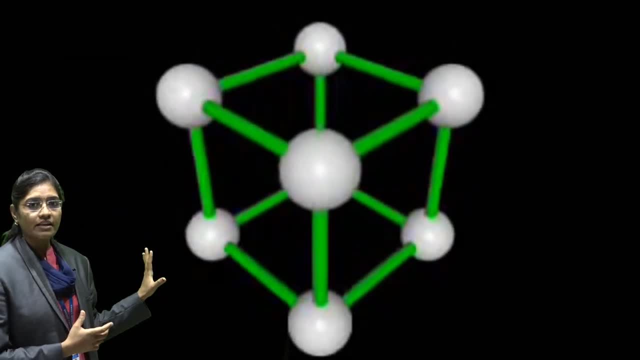 simple cubic crystal structure. see in simple cubic crystal structure. see in this figure, the simple cubic crystal, this figure, the simple cubic crystal. this figure, the simple cubic crystal structure. there are structure, there are structure. there are total eight corners and each corners having total eight corners and each corners having 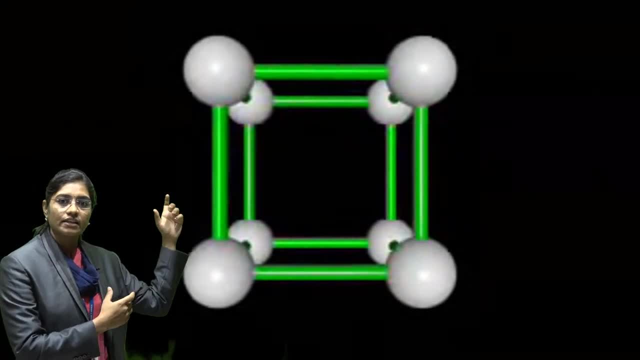 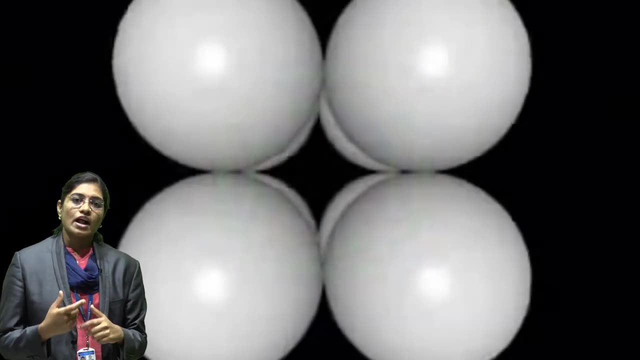 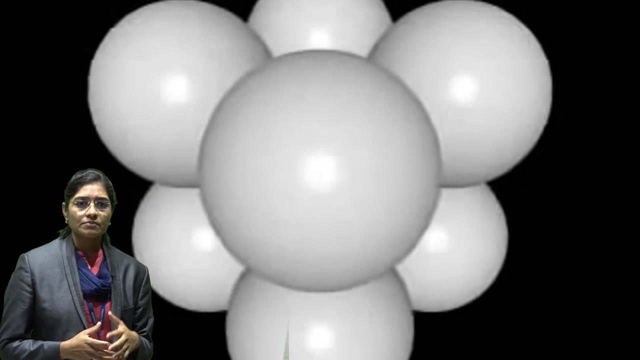 total eight corners, and each corners having eight atoms means here one atom is placed. eight atoms means here one atom is placed at one corner, And in this simple cubic crystal structure the atom is adjoined to another 8 corners of the cube. So here we can say that the number of atoms present in simple cubic crystal 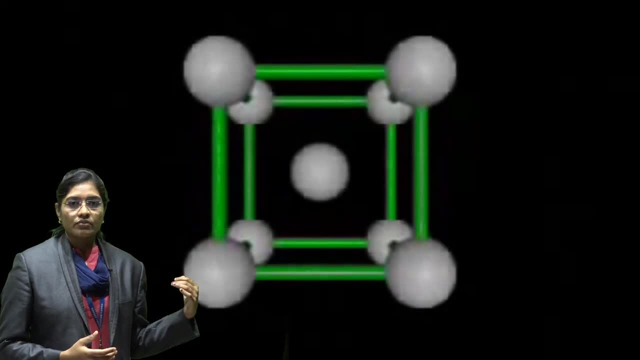 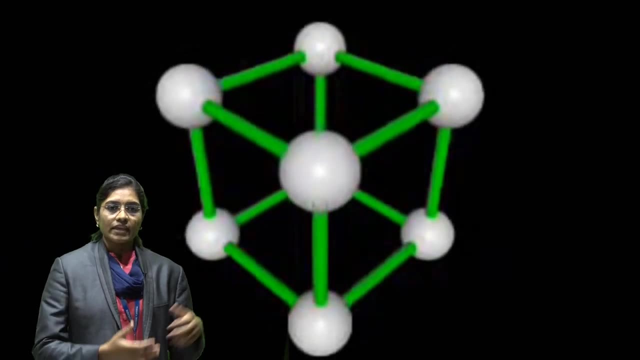 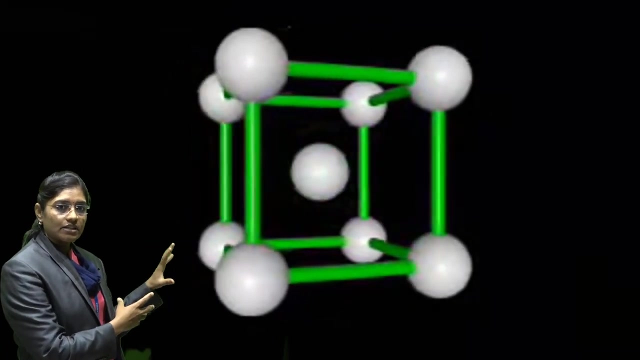 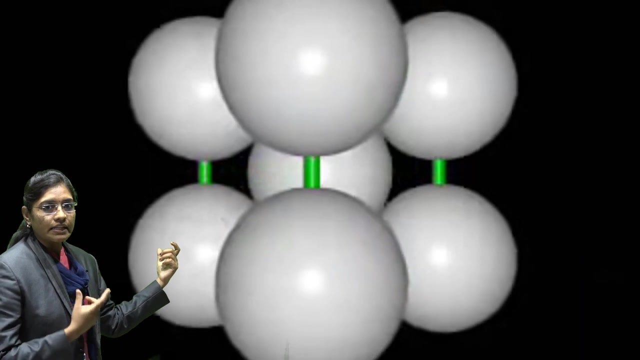 structure is 8.. Now here we take second type of crystal structure is body center cubic crystal structure. Same in this crystal structure, the 8 corners having 8 atoms means the 8 atoms are placed in 8 corners and the 1 atom is placed in a center of a body. So here the number of atoms. 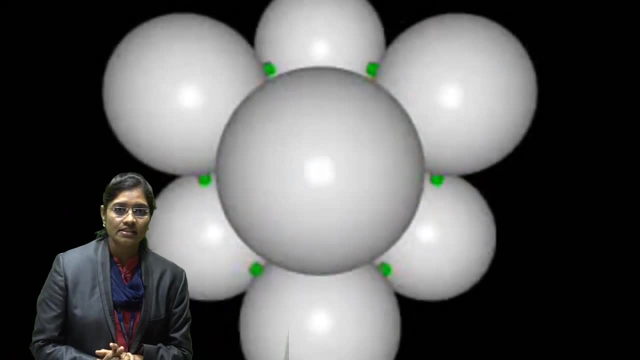 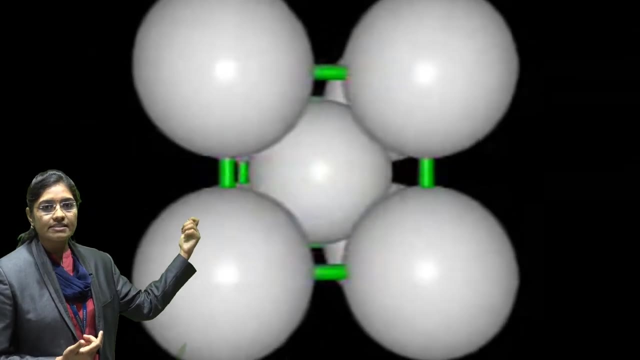 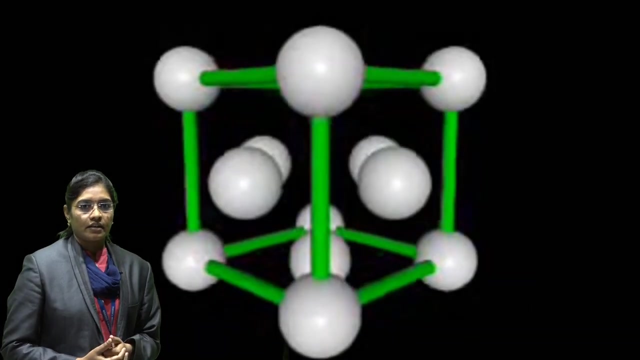 are present in this crystal structure is 9, because the 8 atoms are as in a cube and 1 is placed in a center. So the total number of atoms in body center cubic crystal structure is 9.. Now the third one is a face center cubic crystal.